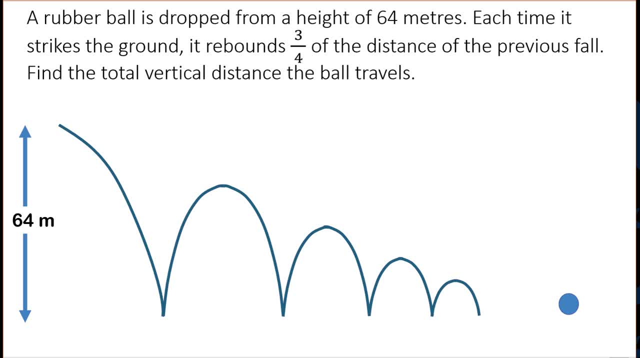 fell, bounced up, fell again, and it just continues like that until it stops moving. now I'm going to break up the motion of the ball, and the motion of the ball consists of downwards movement combined with upwards movement, now the total downwards motion, and I'm only looking at the vertical distance. 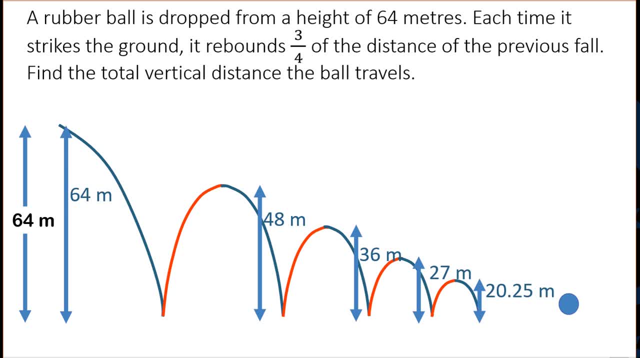 forms a geometric sequence where a- the first term is 64 and R is three quarters 48. that second term divided by the first term, 64, is three quarters. the common ratio there is three quarters. so that's the downward motion of the ball. then in red, 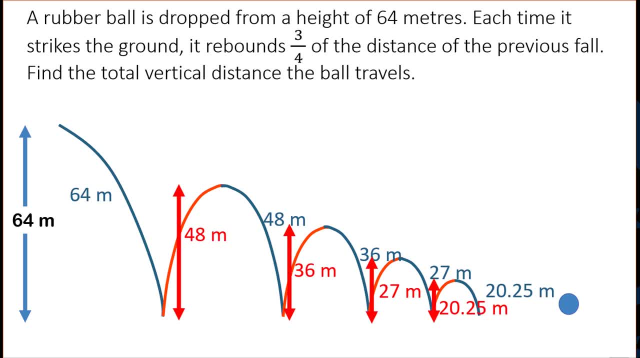 you've got the upwards motion of the ball- and again I'm only concerning myself with its vertical motion, the vertical distance traveled by the ball, and that vertical motion actually can be thought of as existing. well, it's in the form of a geometric sequence where a is 48 and R is still three quarters. 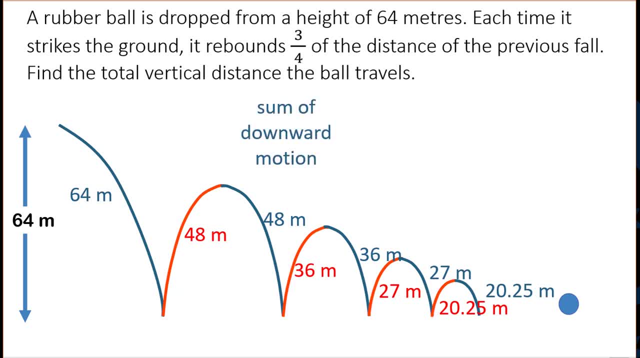 now I'm going to get. the sum of the downward motion, and are being three quarters, is less than one, but bigger than minus one. that means the absolute value of R is less than one. so therefore I can use this formula: the sum of the infinite series is equal to a over 1 minus R, where a is 64 and R is three. 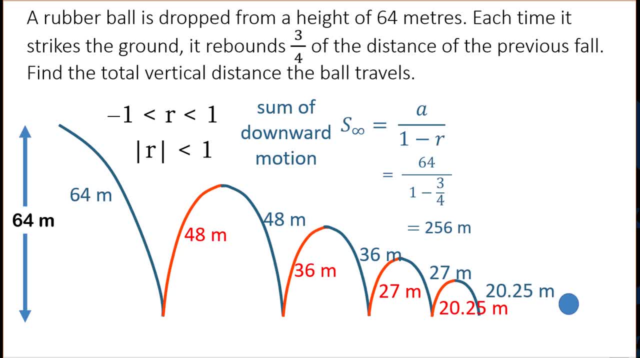 quarters and that works out to two hundred and fifty six minutes worth of downward motion in total. now I'm going to get the sum of the upward motion and using the same formula, with a is 48 and R is three quarters, I get a total of 192 meters of upward motion and I add those two numbers together to get 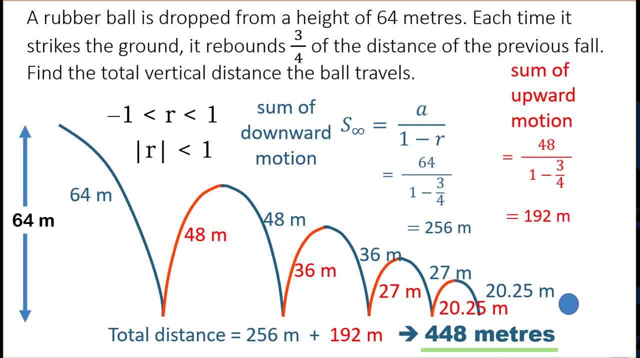 the total distance, and that's 448 meters. that number represents the total vertical distance covered by the ball, and that's the answer to this question. thank you for watching this presentation.